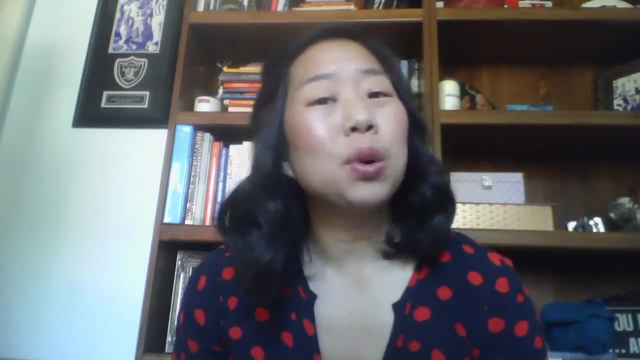 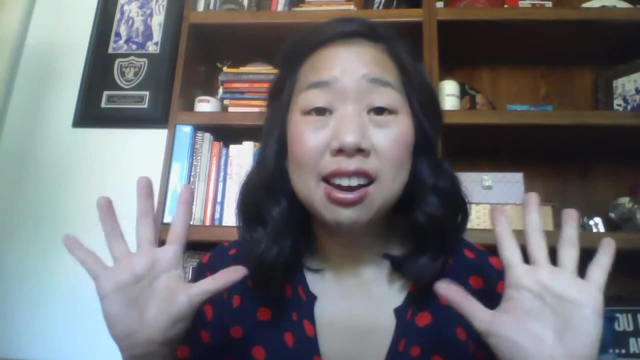 Hello there. If you are a middle school math teacher looking for some hands-on math activities, you are in the right place. If you would like to download 10 free middle school math lesson plans including several of the activities that I'm going to be sharing with you. 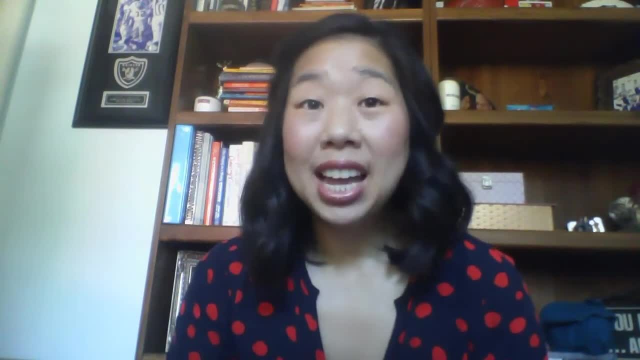 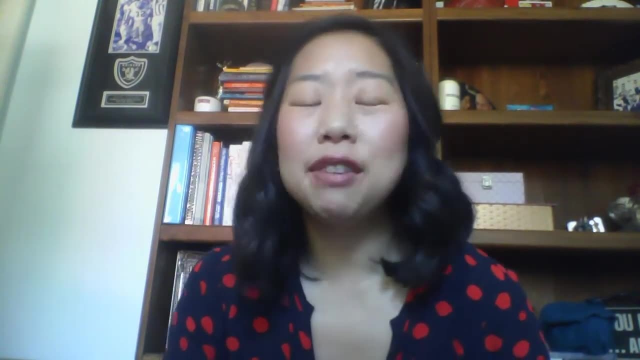 click the link right below in the description and go ahead and download your 10 free middle school math lesson plans. If we don't already know each other, my name is Kathy Martin and I'm the creator of the Pre-Algebra Teachers Middle School Math Membership. We are your. 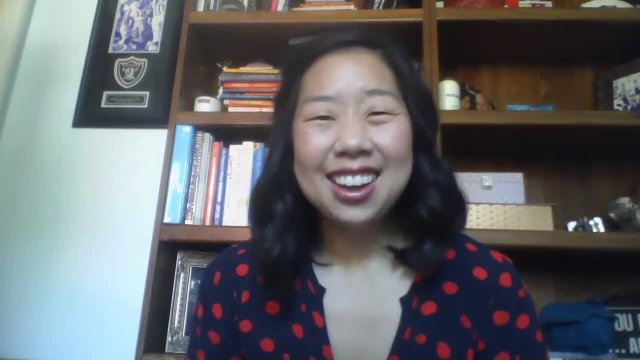 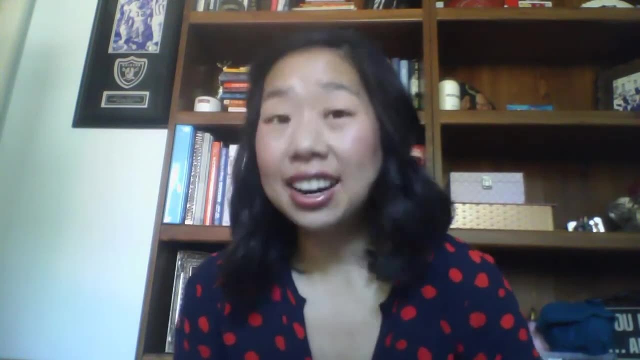 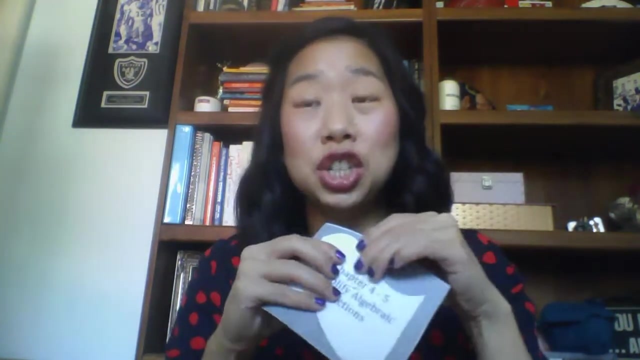 one-stop shop for everything you need to teach middle school math. Today, I want to share with you my favorite hands-on middle school math activity, and that is task cards. Task cards are printable cards just like this, and I love using them because there are three particular ways that. 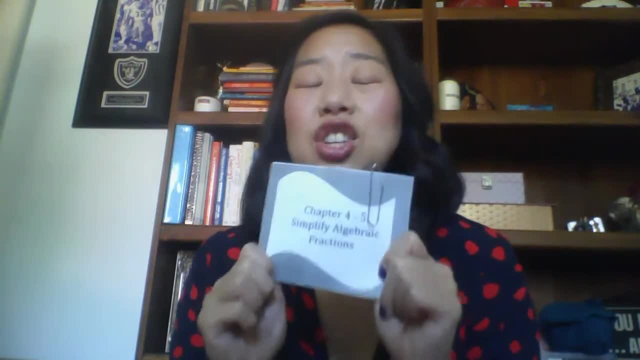 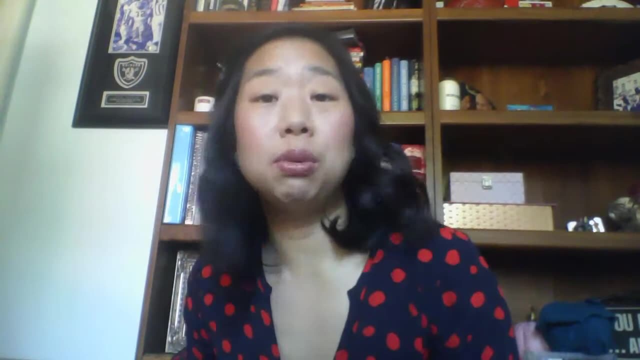 I love using them. that really make it easy for me to learn. I love using them because they're big task cards- amazing. But before I tell you about that, I get so many questions on how do I store task cards and I just want to share with you that I have a container like this. I got it at 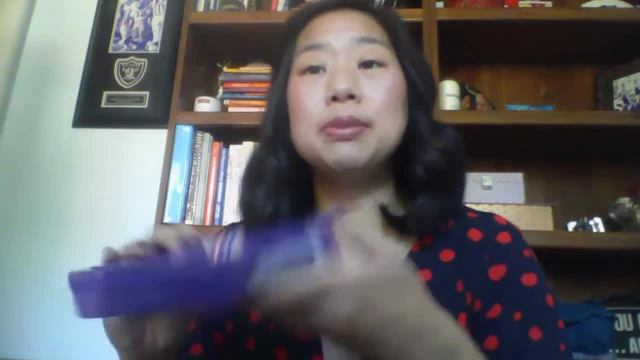 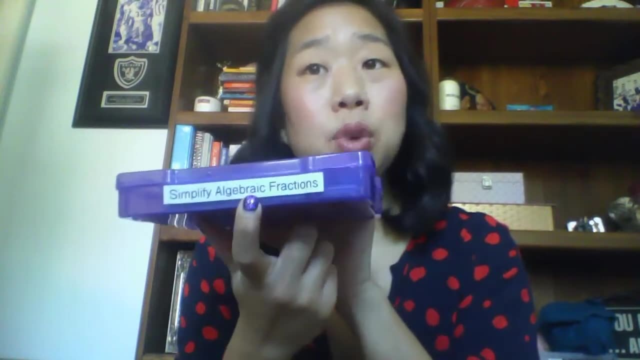 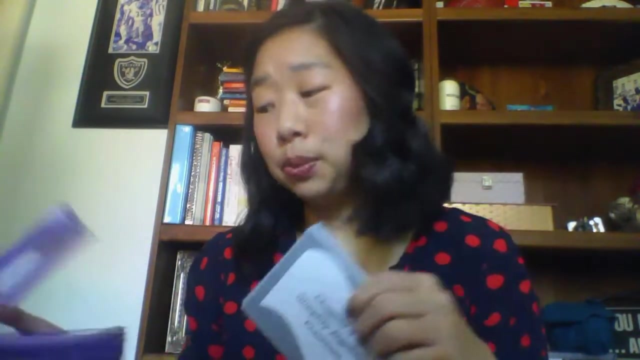 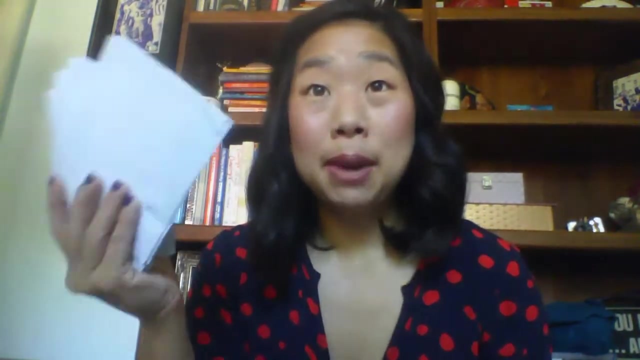 Michael's, and when you open it it comes with these plastic containers like this and I just use a label maker and label what each one is. So this one is Simplify Algebraic Fractions. So I get so many questions about how to store them because it can be a lot Like when you have piles. 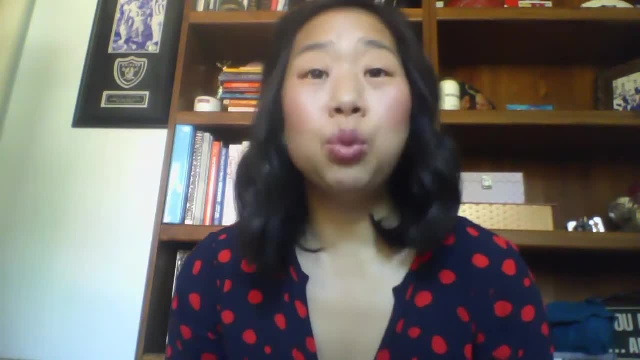 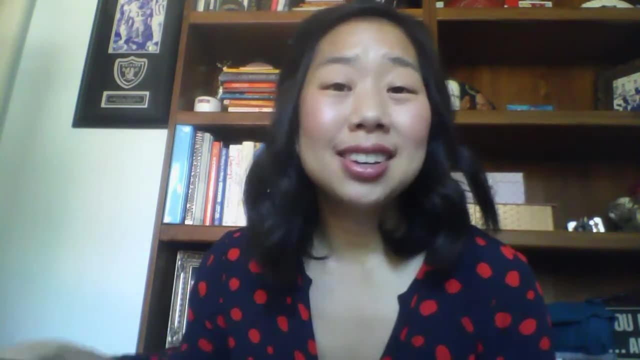 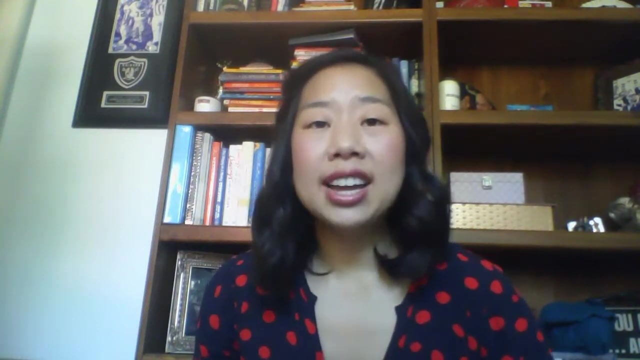 of paper, like stacks of paper, like this, it's hard to keep track and we want things to be organized, easy to find and easy to access. So, Michael's, and there's always coupons, there's always deals, so wait for a special. Okay, so let's talk about why task cards are amazing. 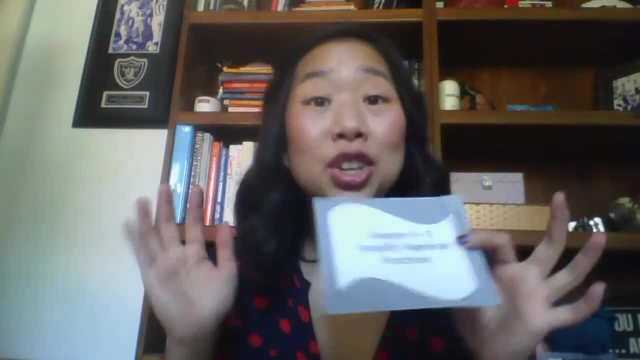 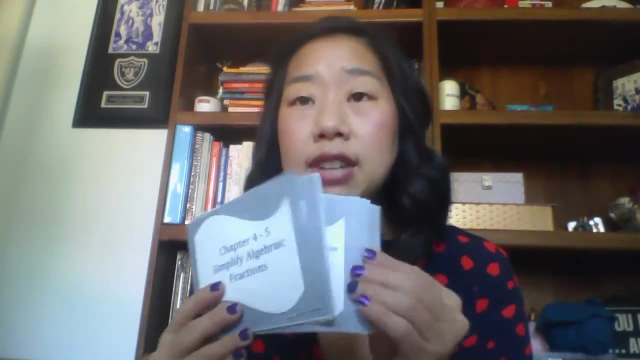 why I love them and why I love them. So let's get started, So let's get started, So let's get started. So let's talk about why I love them as a hands-on activity and why you really should be incorporating task cards in your classroom. So the first, so my set of task cards includes 15. 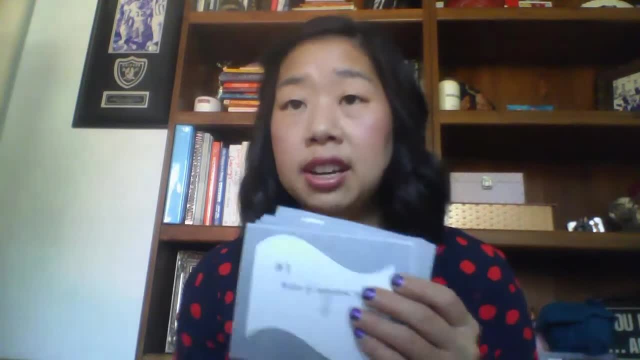 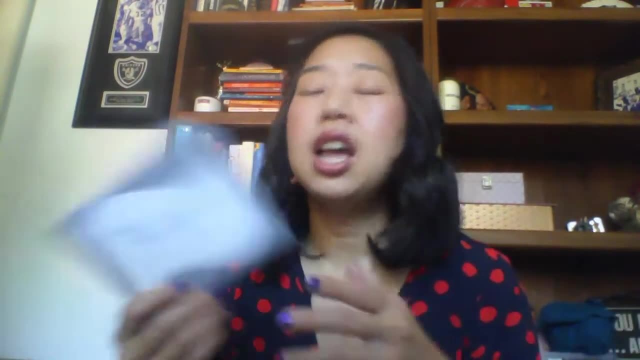 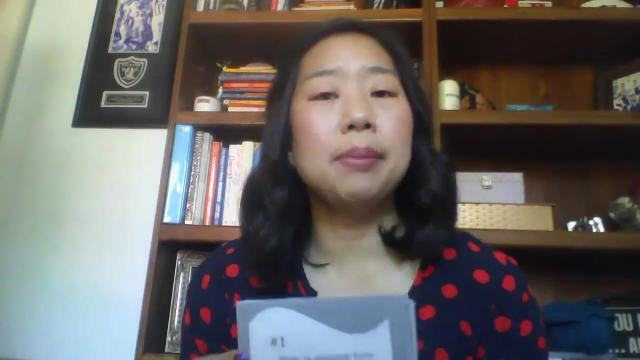 questions and I love this. I love task cards because if you have students who get overwhelmed by a worksheet of like 30 questions, these are great, because there's only one question on a card, So you're working on one question at a time. 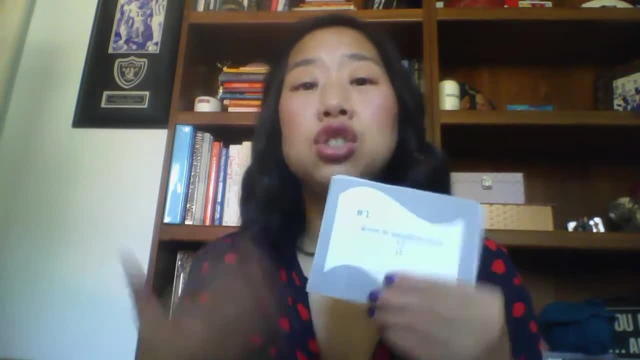 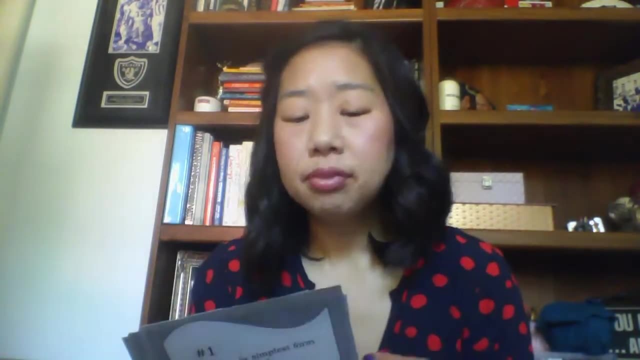 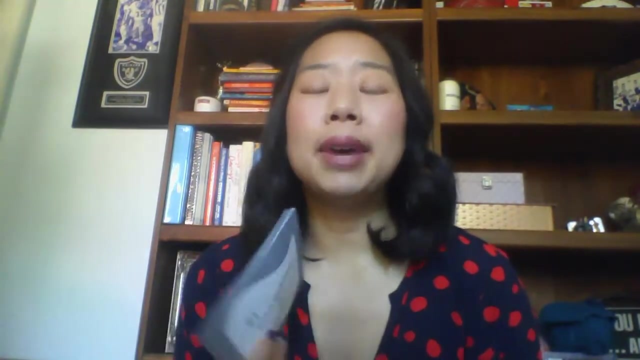 Kids feel a lot less overwhelmed. They feel like they can actually do the problem and it just seems easily attainable, right when you're just working with one question at a time. So, with that being said, I love using these as a homework alternative. So, instead of giving my 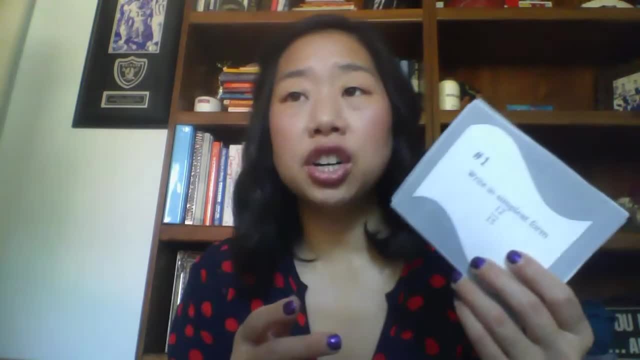 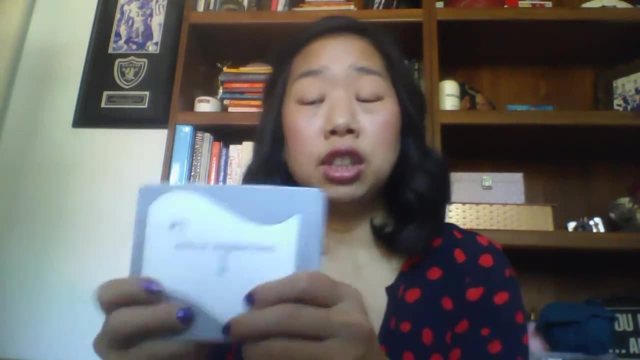 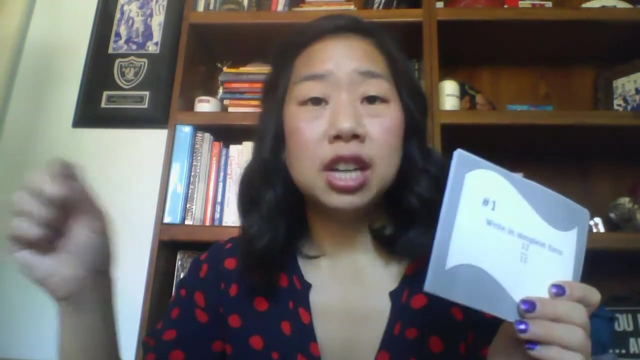 students a page of 20 questions. I give them these task cards and I know that there's 15. I don't always assign 15. You can use. you can certainly give all. give your students all of 15 questions and have them do all 15.. We have a template where students use a template to show. 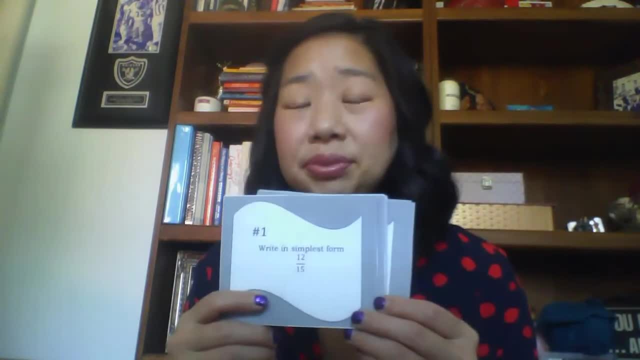 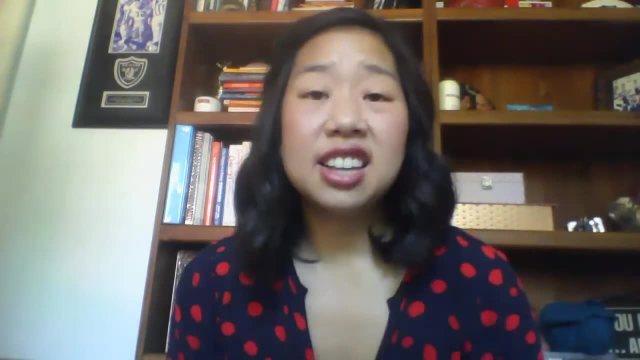 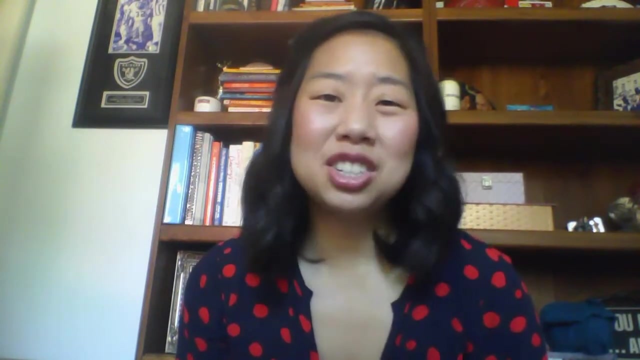 their work and write out the problems. Or I sometimes like to give my students the power of choice and let them give them the whole stack of 15 and say, hey, pick 10 of them to do any 10 you want, And they can kind of go through and see what they want. Most of my students just 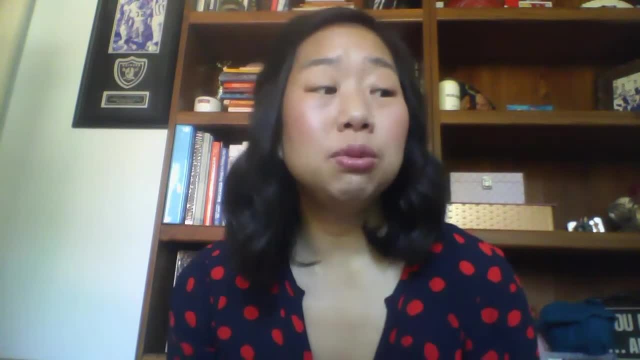 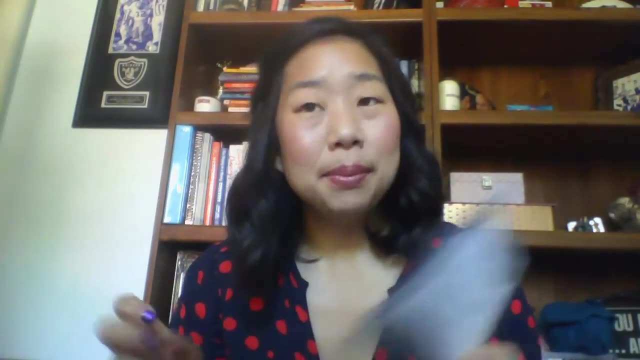 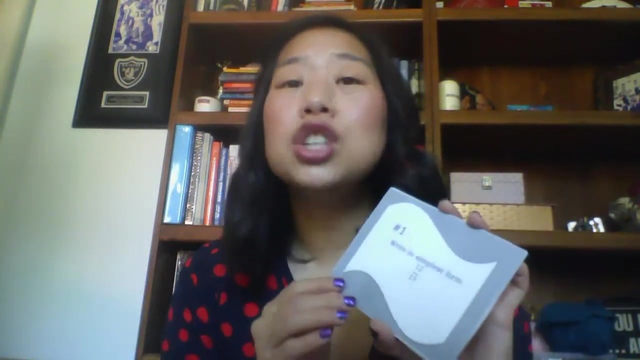 do one through 10, but it does give them the opportunity to decide And, um, that is also very powerful. So homework alternative um number two reason why I love task cards and why they are an amazing hands-on activity is to use them in small group. And what's even better, 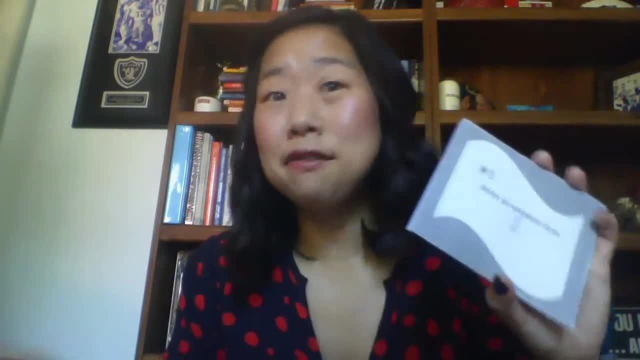 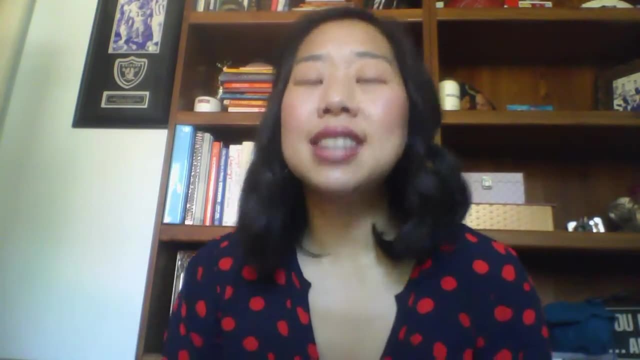 about using them in small group is you only have to print out like five or six sets, because your small group- at least my small groups- are no more than six kids. really, even six kids is kind of pushing it, But then I, you know, only can have six Like. 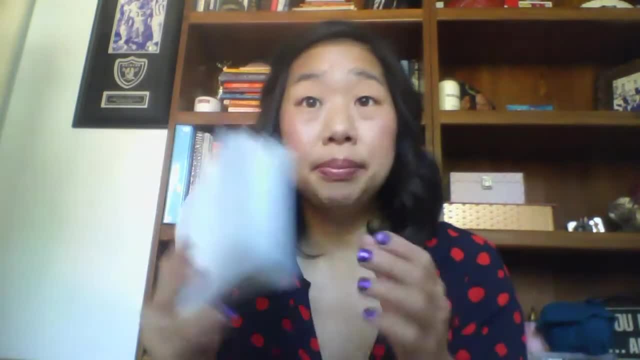 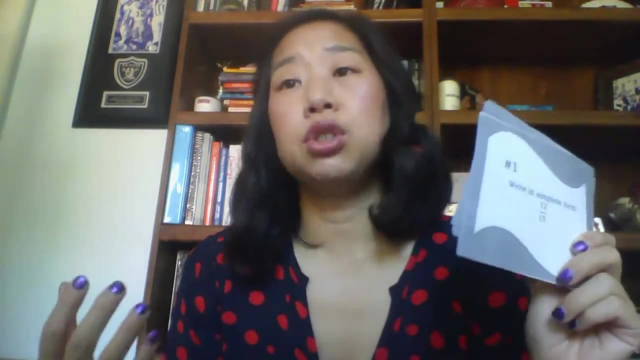 I only need to print out six sets. in this particular box I have eight of them, So using them in small groups really, really helps. And it's the same thing: when you're working in small groups, you can have students do all 15 or pick six of them for, have six of them for them.